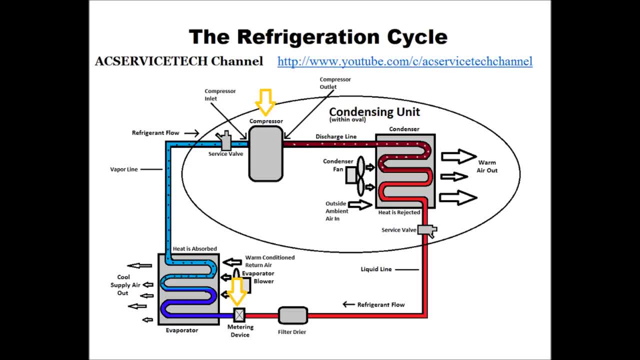 on this system, And the one is the compressor that's up high, and then the other is the metering device where, in this picture you see, it's down low. Alright, so how the refrigeration cycle works is it takes low pressure, low temperature vapor refrigerant it comes into. 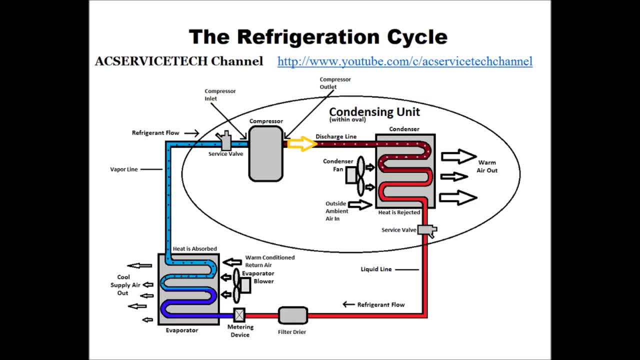 the compressor and out of the compressor it comes out as a high temperature, high pressure vapor refrigerant. In fact, it's at its hottest spot on the entire system right there. As it enters into the condenser coil, it starts rejecting heat. As it rejects heat, it starts. 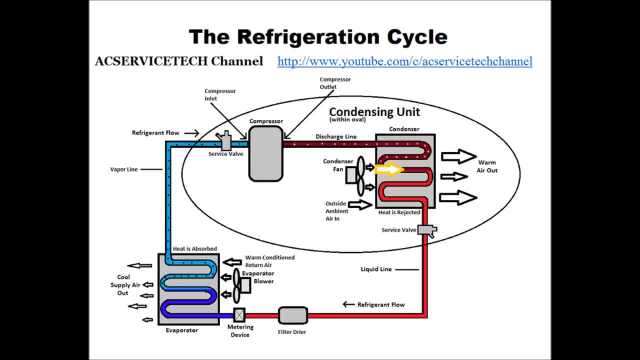 turning into a saturation. The saturated state is where vapor and liquid both exist at the same time. Alright, so right there, right after the saturated state where it turns into a complete liquid, until where it comes out, right next to the service valve, the temperature decrease as it's rejecting. 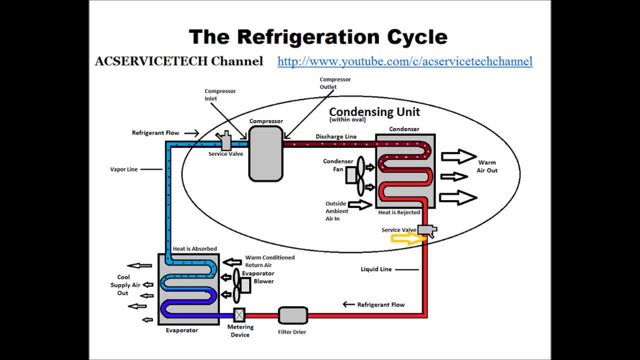 heat. the temperature decrease in liquid form is called the subcooling. Alright, the saturated state is where the vapor and liquid both exist at the same time. Alright, so right there it's at its hottest spot on the entire system, right there As it enters into the compressor. 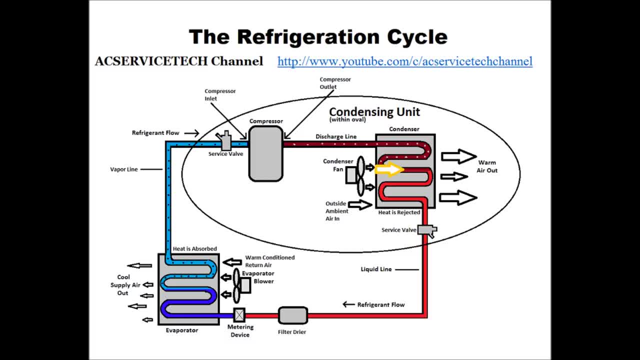 it's at its hottest spot on the entire system. right there, Alright. so right there, the refrigerant is where it's transferring most of its energy. at Alright, the refrigerant is what is carrying the heat and moving it, rejecting it and absorbing it in the refrigerant. 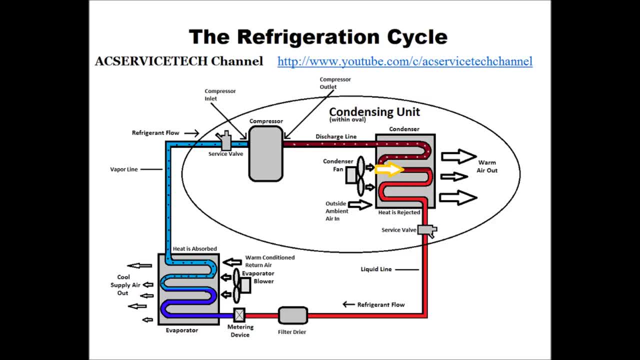 itself And most of that energy transfer occurs right in that saturated state. Alright, so it comes from the saturated state in the middle of the condenser coil. it continues to reject heat as a complete liquid until it comes out of the condenser coil. Then it 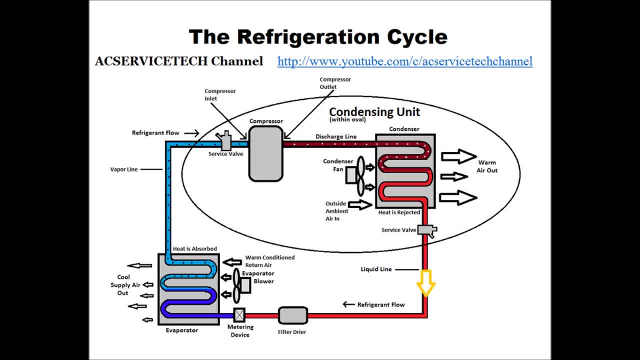 comes down in the picture here and then it makes a left and then it goes in through the filter dryer. The filter dryer is there to absorb any moisture in the system. Alright, it has a fixed capacity and that's it. Alright, it comes through that and then it hits the 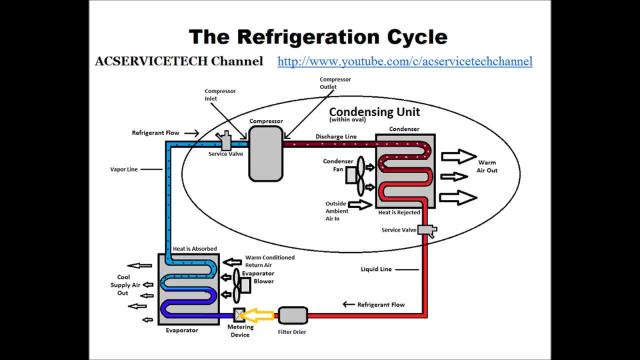 metering device. The metering device allows for a pressure change. Alright, when you have a pressure change, so you have high temperature, high pressure liquid refrigerant coming into the metering device and then it turns it into a low pressure, then what happens is: 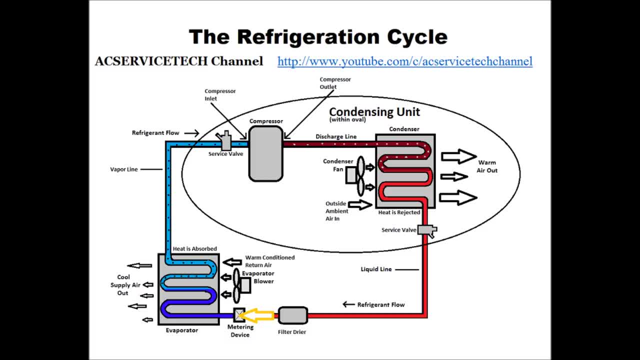 it automatically Makes it a low temperature as well. So if you decrease temperature, then pressure will decrease. If you decrease pressure, then temperature will decrease. So in this case we have a high pressure, high temperature liquid refrigerant coming through and hitting the metering device. 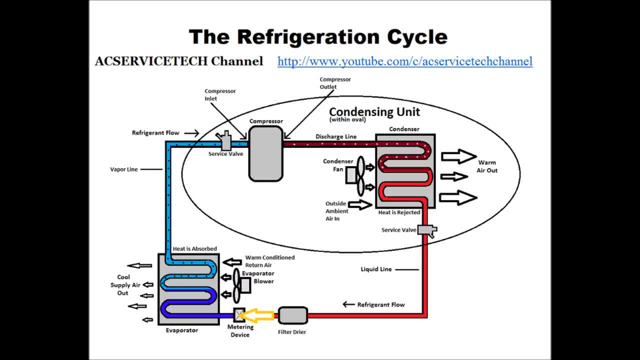 The metering device is only going to allow a small amount through, Alright, and then it turns into a low pressure, low temperature 80% liquid, 20% flash gas mix. But it's mainly going to be a low temperature, low pressure liquid, Alright, until it gets to the middle of the evaporator. 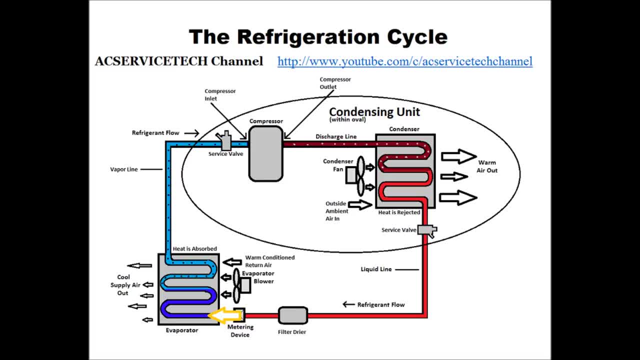 coil. So the refrigerant is actually absorbing heat once it enters into the evaporator coil. As it absorbs enough heat, it turns into that saturated state in the middle of the evaporator coil, alright, where most of the energy absorption is taking place. and then right after that, 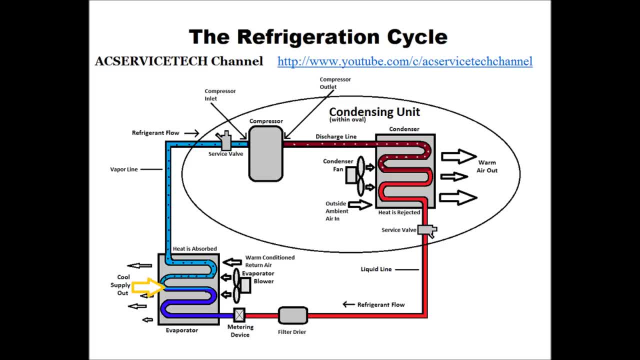 is where it turns into a low pressure, low temperature vapor: Alright. right after the saturated state it turns into that low pressure, low temperature vapor alright. until where it comes out of the evaporator coil. it's still absorbing heat As it comes out of the. 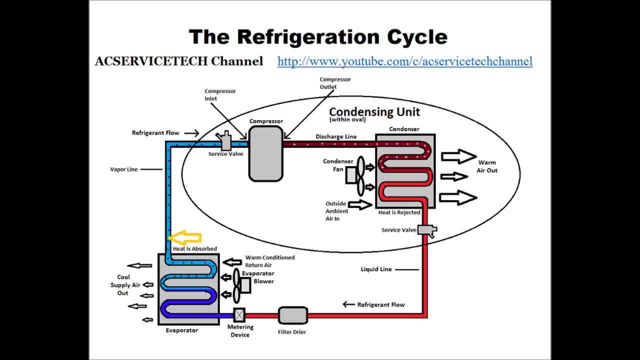 evaporator coil. right at that point, right there the temperature increased from the saturated state in vapor right at the end of the saturated state in vapor to where it comes out. that's called the superheat. If you continue along, you keep coming up. 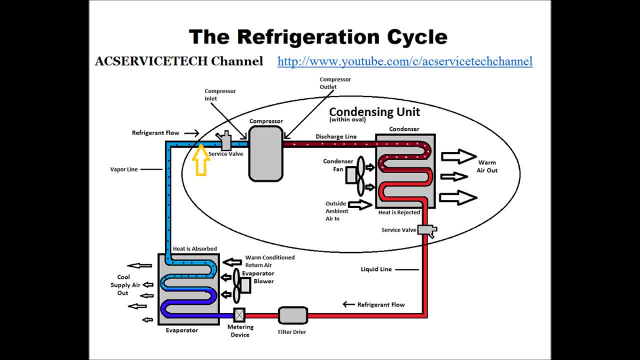 as a low pressure, low temperature vapor. you come up and then you make a right and then you come back up And then you come over to the service valve. Alright, so that's where we take a superheat reading at, Alright. so if you took right in the middle of the evaporator, coil right. 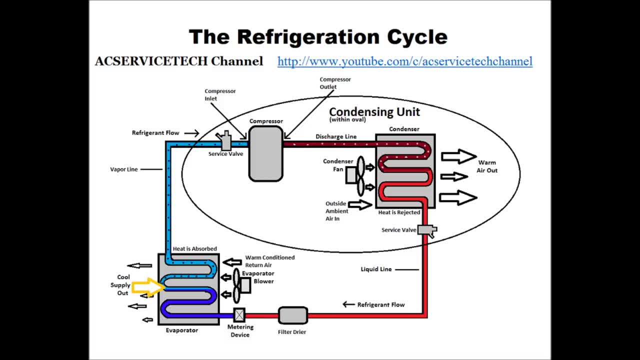 after the saturated state where it turns into a complete vapor, the temperature increased from there all the way over to the service valve next to the compressor. that's called the total superheat. Alright, after that it just enters back into the compressors. a low. 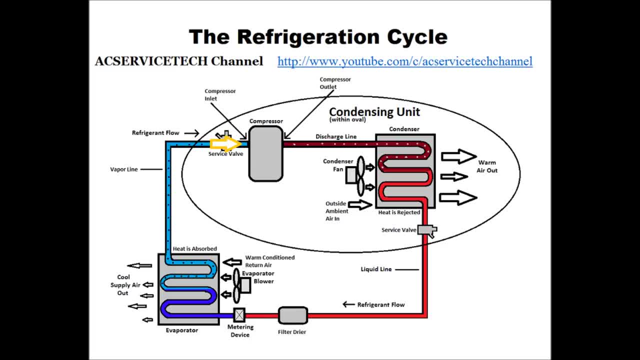 pressure, low temperature vapor refrigerant and the refrigerant cycle starts all over again, Alright, well, I hope you enjoyed yourself and we'll see you next time at the AC Service Tech channel.